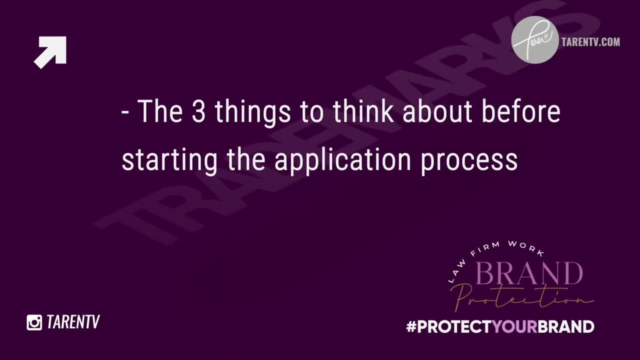 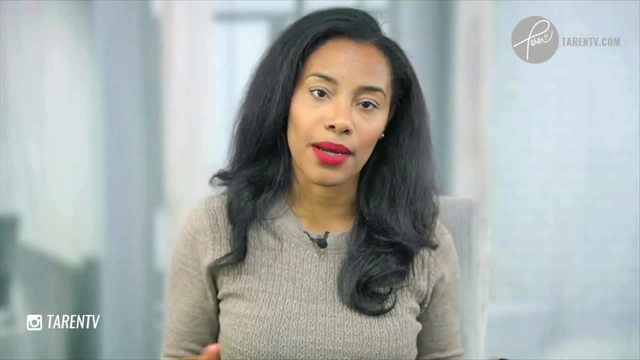 walk you through the three things that you need to kind of be thinking about before you prepare that application or retain your lawyer. Now, some of you will attempt to file your trademark on your own. I do not recommend this, because trademark lawyers know how to. 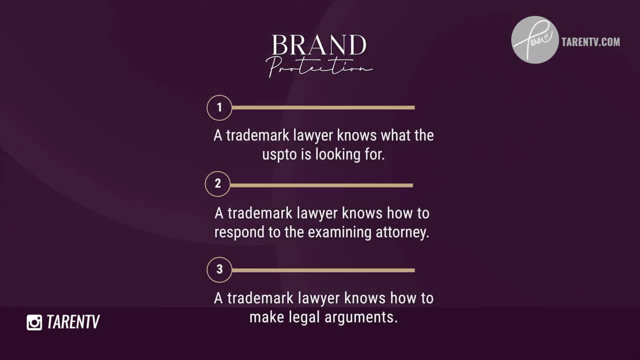 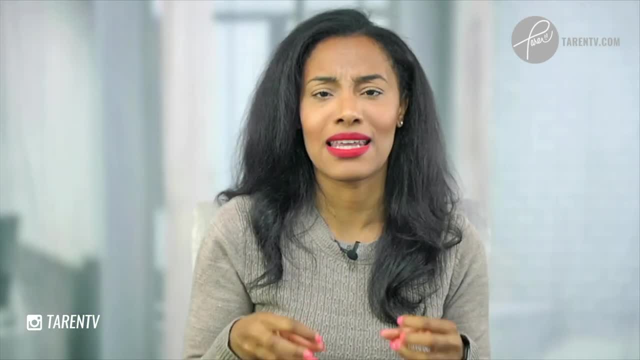 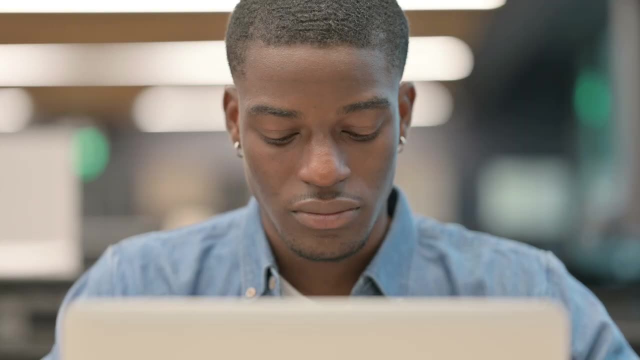 properly classify, submit, describe research and make arguments on the application to get your trademark A approved and B limit the office actions. If you guys are not sure what office actions are, let me explain to you how the trademark process works So obviously. 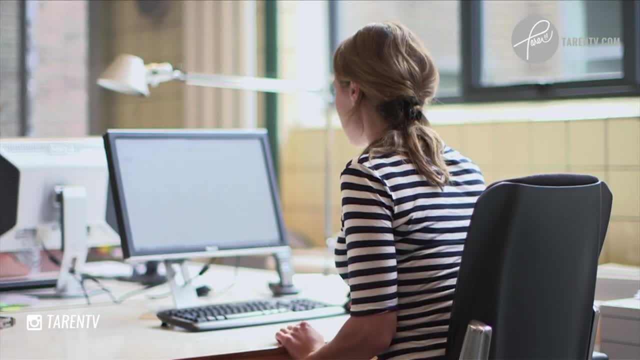 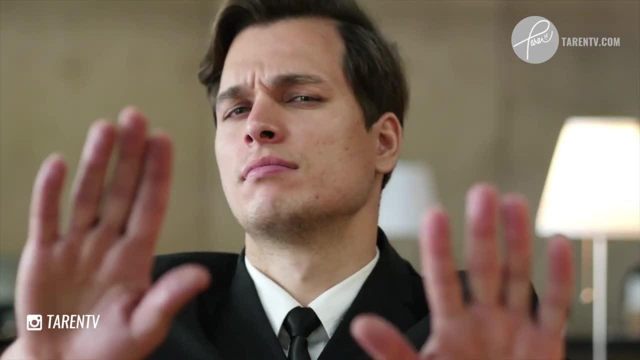 you guys can go online and you can look up stuff. Most people that come to me they say: oh, I already looked it up and I know that my trademark doesn't exist, because I typed in my exact words and nothing came up. That's not thorough. 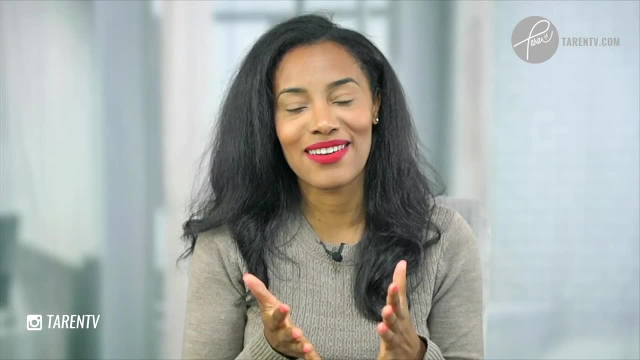 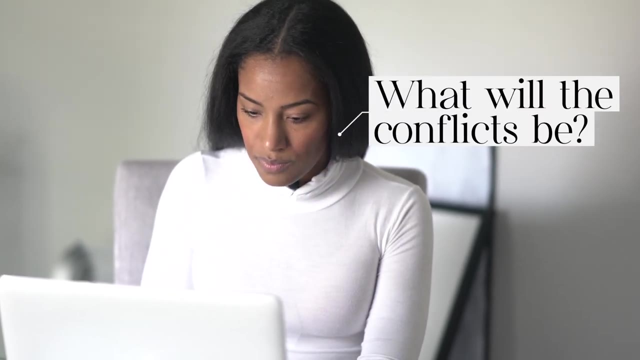 I have done my own research on a trademark and that is not what a lawyer is going to do. They're going to go really deep into the research process to figure out whether or not your risk is high or low on your mark and just kind of figure out all of the dangers. 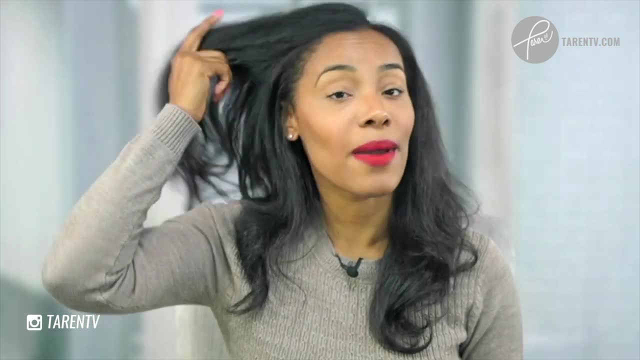 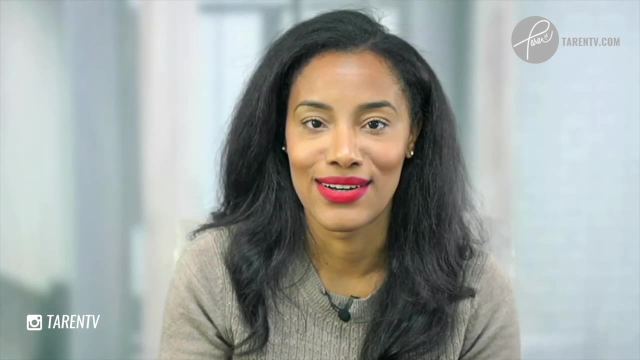 that are out there with your trademark, And the thing that you really want to pay attention to is this thing called office actions. So when you're filing a trademark, you are starting a legal process. This is not just a paperwork or application that you submit to this office. where there's no legal process. This is an application that you submit to the office and you're going to file it and you're going to look into it. So the legal process is going to be a process that you complete in the office. You're going to want to do a legal process. 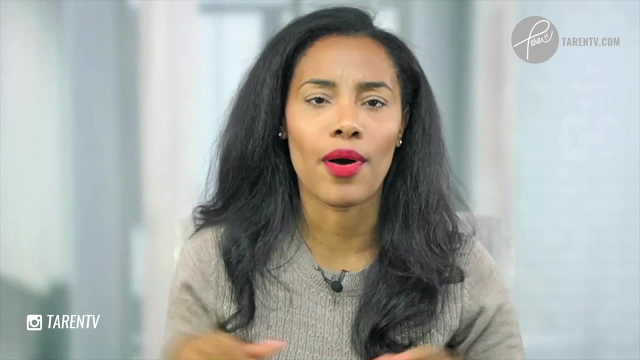 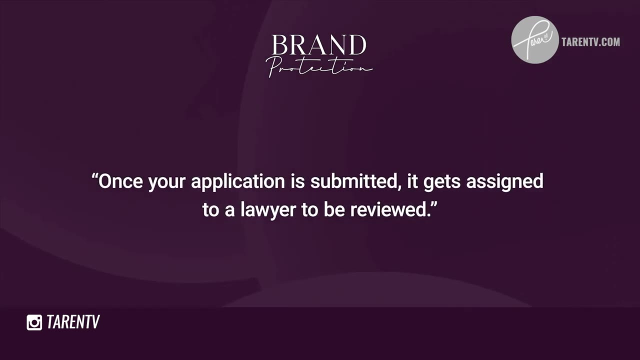 of this process. You have to give it a lot of time and a lot of time and a lot of time and a lot of just a whole bunch of administrative people, kind of checking off of a database. what happens with the trademark is that once that application is submitted, it goes to a set of lawyers. 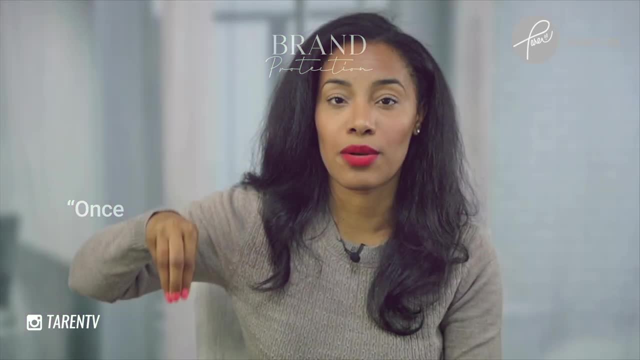 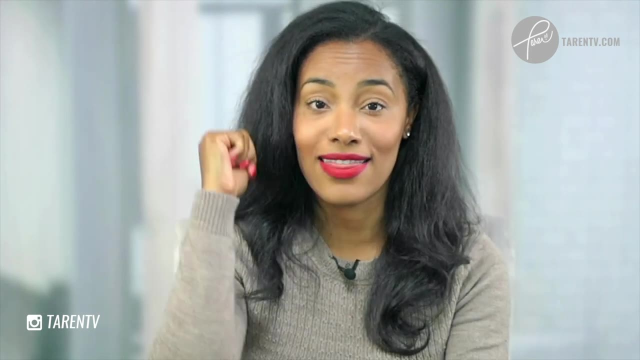 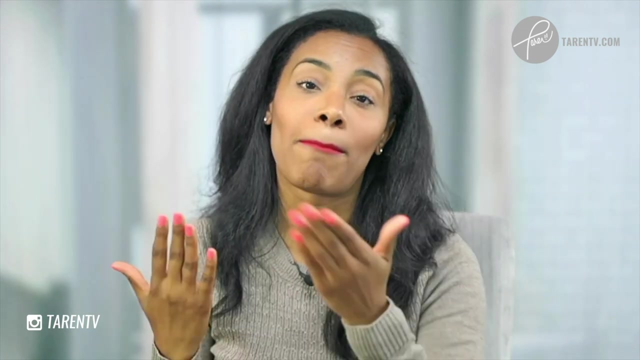 lawyers who are working to make sure that everything inside of the trademark registration or registry is going to be protected. so their job is to make sure that their proverbial clients, the people who already have registrations, are not going to be offended or conflicted by what it. 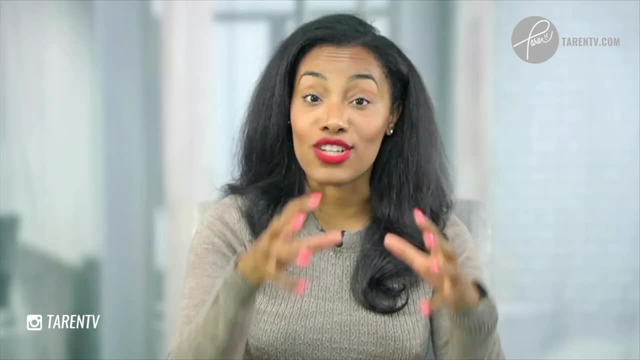 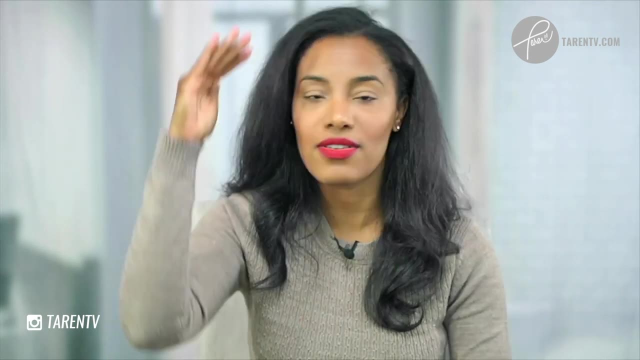 is that you submit so an office. action is when that attorney that's assigned to your trademark goes through the database. they look up things and they're like, oh, hold on, we found all these reasons why we don't think your trademark should be able to pass through, and so they will send you. 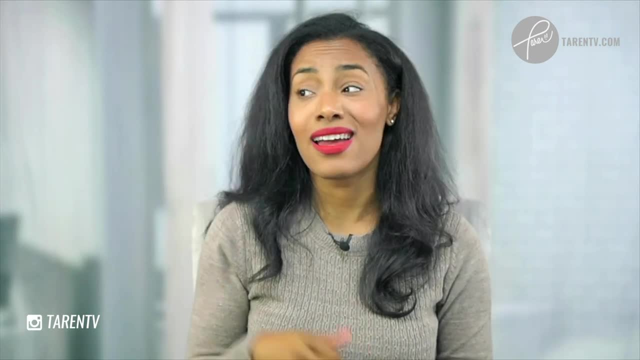 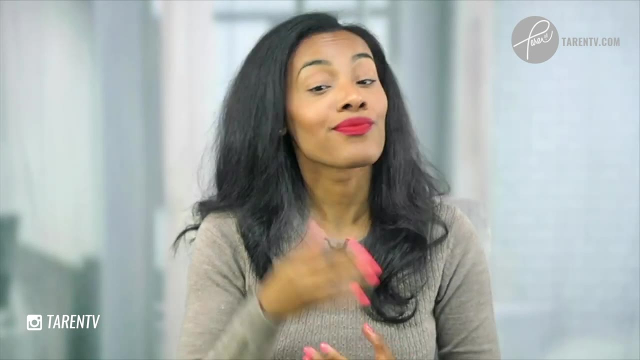 back a list of things that you have to do in order for them to say: yeah, no, we're not going to do it, it's going to conflict with these other registrations. or they'll say: if you can make this argument- and you can make it based on the. 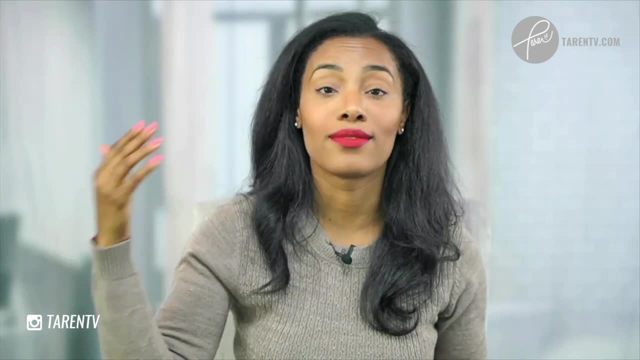 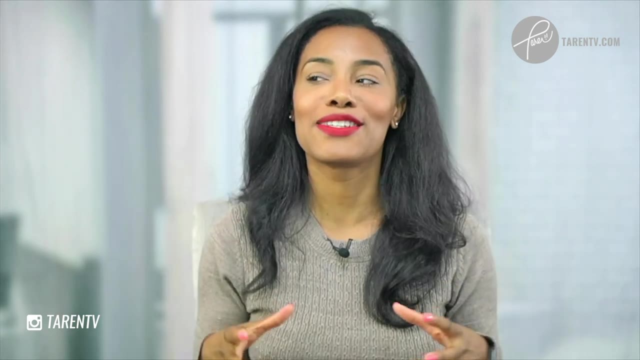 case law that we need, and you can make it based on the. you know the laws that are already established that keep you from getting this in. we'll give it to you, and so that is what the beauty of having a lawyer file your trademark is is because we already know what these people on. 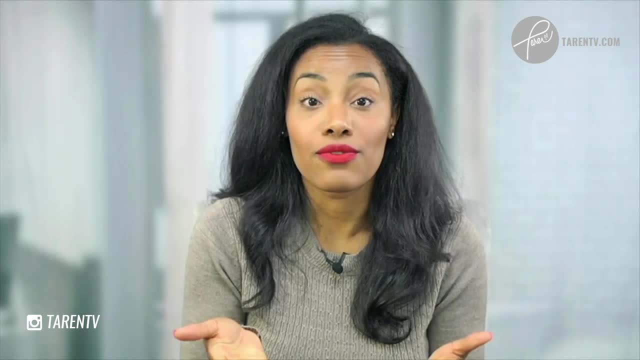 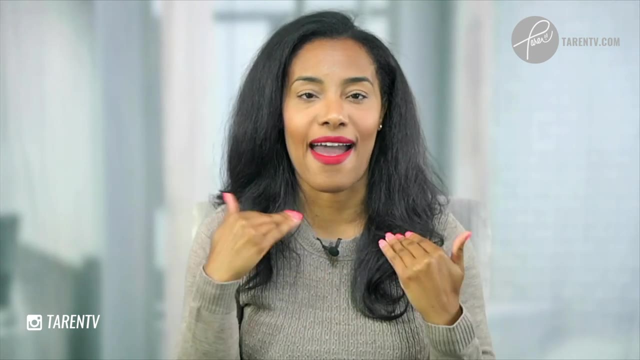 the other side, these other lawyers at the uspto are looking for. we're looking, we know what they're watching for when it comes to a trademark, and so we know how to argue. if they come back and they're like, we know how to respond and say: 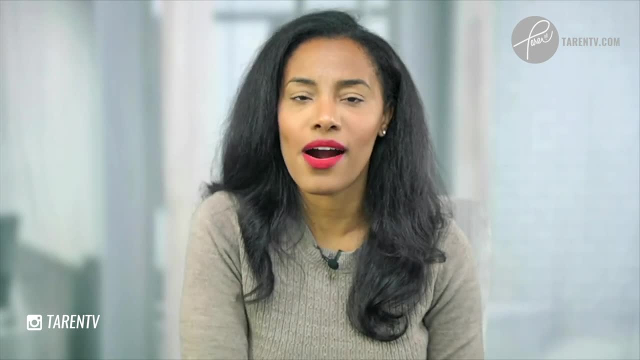 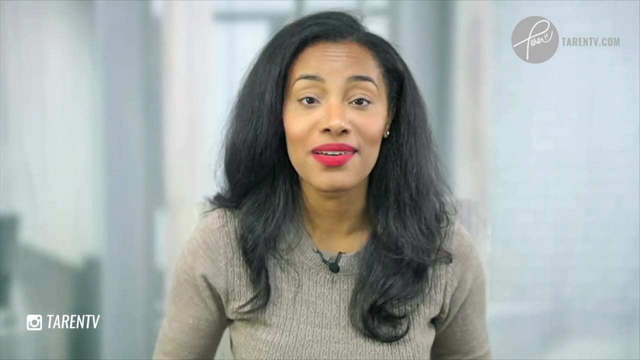 okay, let's try it this way, and we will make a legal argument for why this thing should or shouldn't be so. if you guys are willing to go toe-to-toe with a lawyer, um, that's up to you. i wouldn't recommend it, but that is essentially, in very common layman terms, exactly what happens when you. 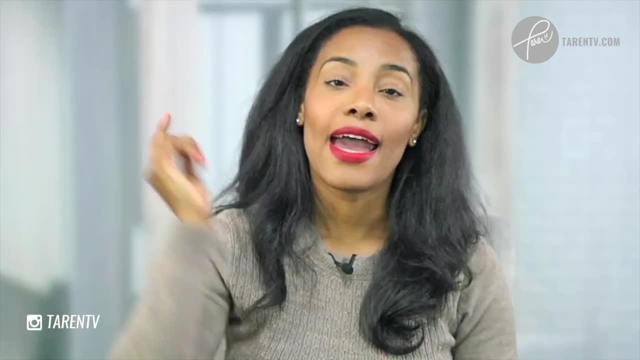 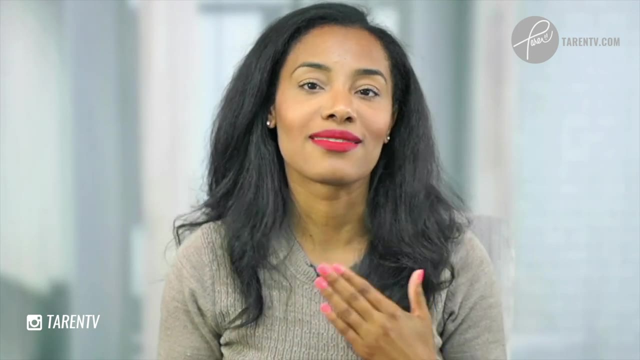 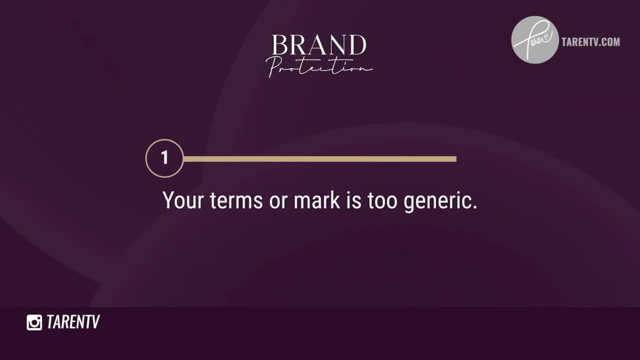 submit your trademark application. let's get back to this video, and now i'm going to break down three really simple mistakes that a lot of people make often in their trademark process. that makes a lot of sense, so let's start with trademark mistake number one. if your terms are too generic, 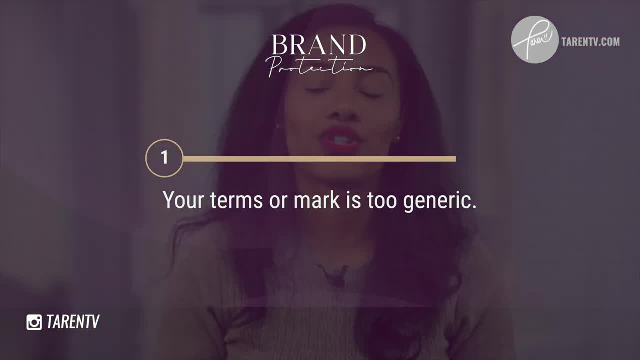 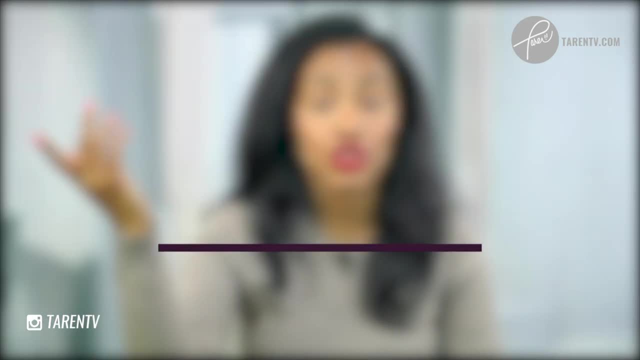 you cannot own or monopolize the english language, and so what the trademark office is going to look for is something called distinctiveness inside of your mark, like in a hypothetical situation: maybe you own a mexican food restaurant and you have these delicious fajitas and you want to get them. 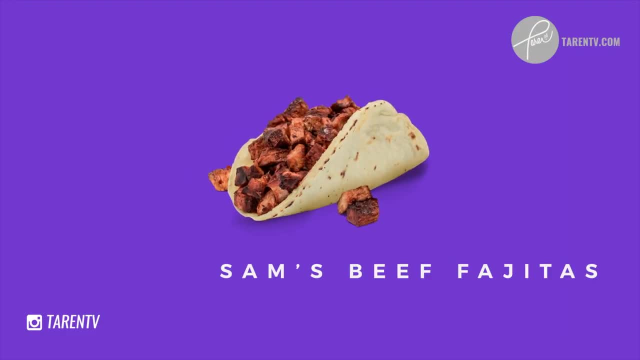 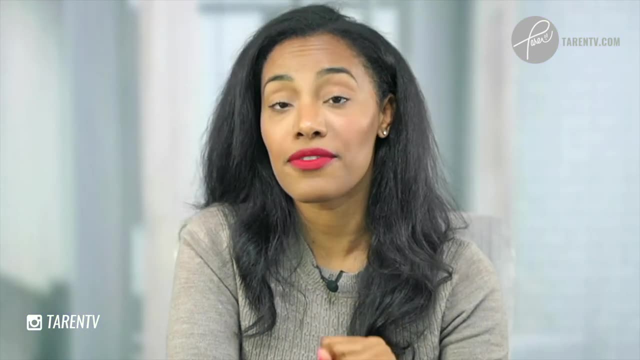 trademarked. and so you're going to say this menu item we are calling sam's beef fajitas, send it off to the trademark office, let's get it trademarked. what i believe is going to happen is the trademark office is going to look for any generic terms. 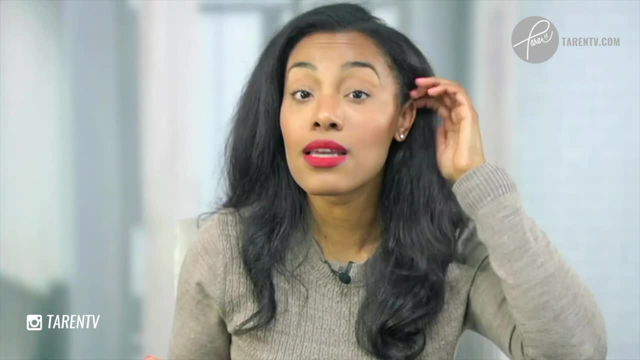 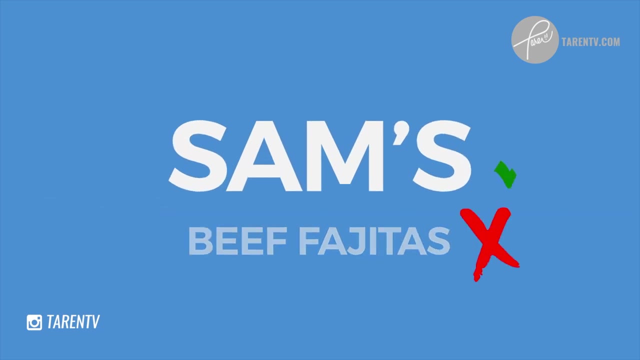 terms that we use to just in general describe things, and in this case, beef fajitas. everybody knows what beef fajitas are. it's not something that you can own or trademark, and so the only thing that's distinctive is sam's- sam's beef fajitas. the only thing distinctive is sam's. 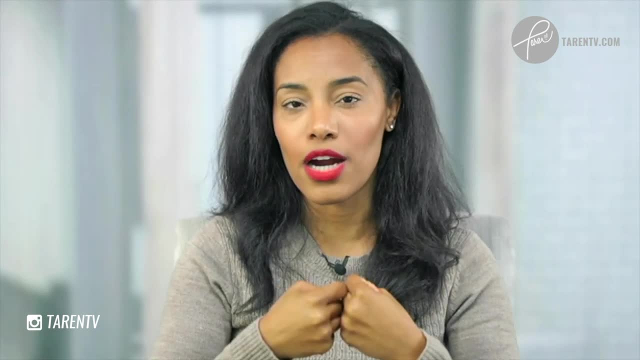 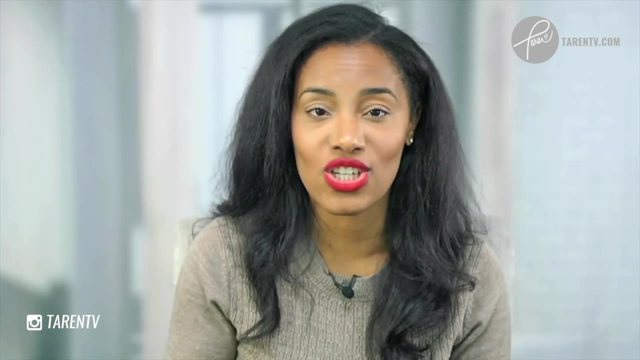 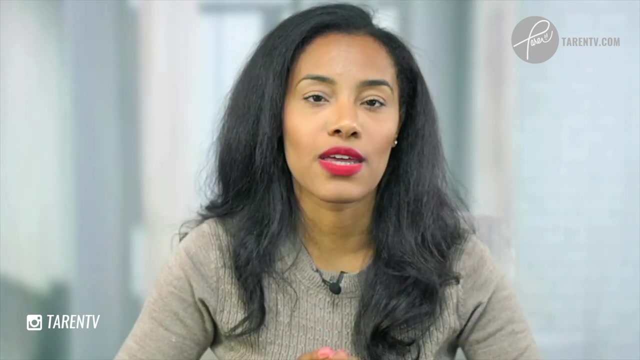 so what i want you guys to think about is how your mark plays into the bigger picture of the english language as well. if your terms are too generic, you need to add some distinction in it so that it makes your mark stronger. now there's other things that are that you kind of have to think about when you're thinking about. 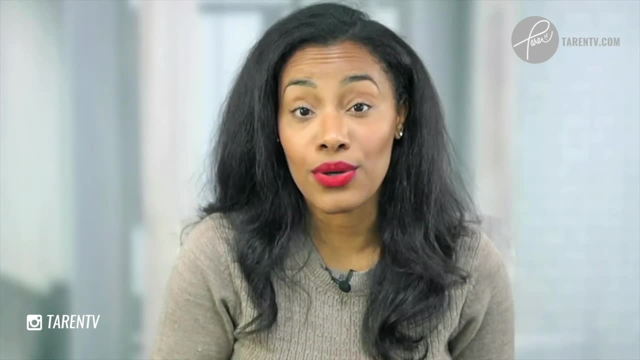 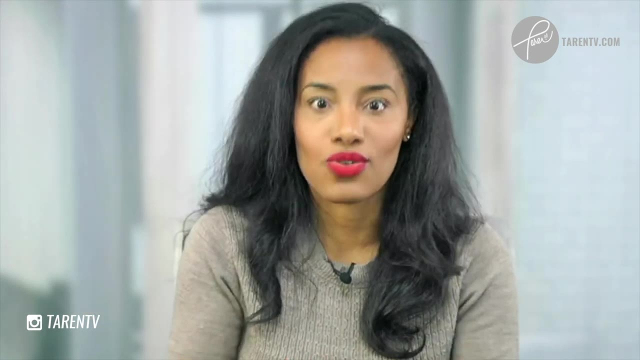 like common terms, like beef fajitas, is how they're being used, because in that particular hypothetical that i just walked you through, we're talking about a mexican food restaurant, so of course, beef fajitas, describing beef fajitas, that's common. now let's think about something. 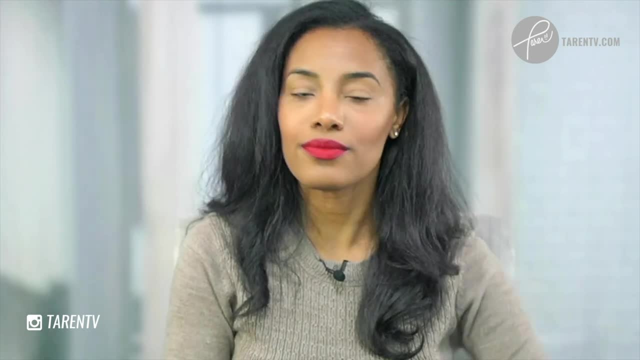 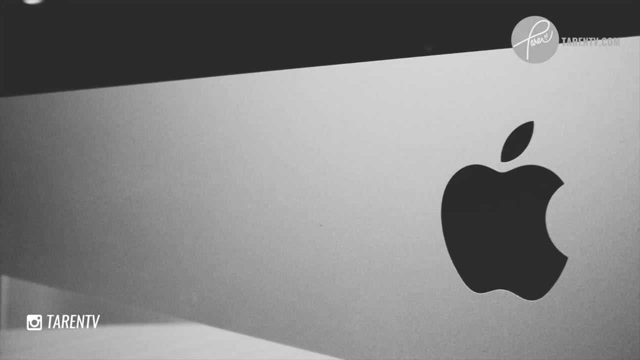 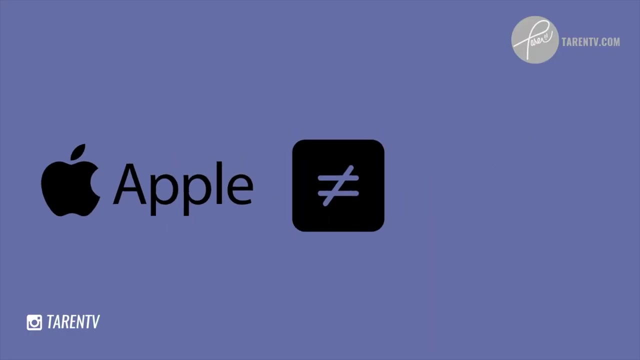 that's not so common. that's very popular apple now. we're not talking about alice's country. red apple is to describe a red apple. we're talking about apple computers, now a very common term. apple is not used commonly and the application makes it distinctive. it makes it a word that you can now. 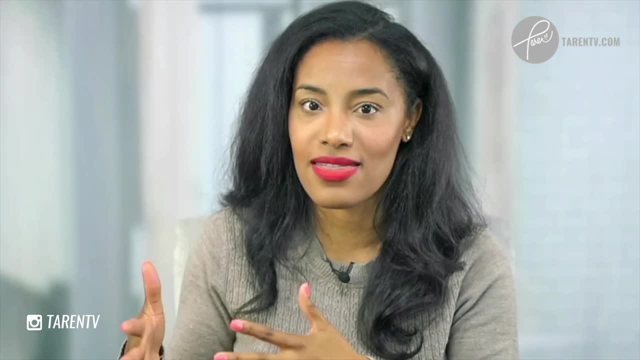 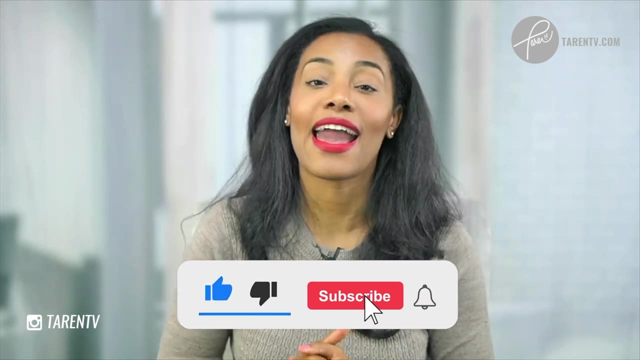 trademark because you're not using it to describe the exact thing that the english language describes make sense. if you guys are finding this information valuable, please hit the like button and don't forget to subscribe and hit the bell so you'll be notified when i post more videos, just like this. 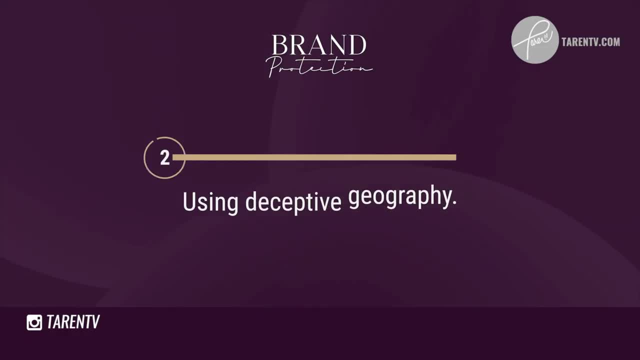 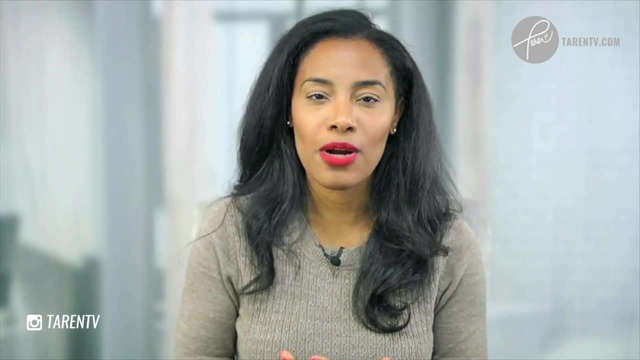 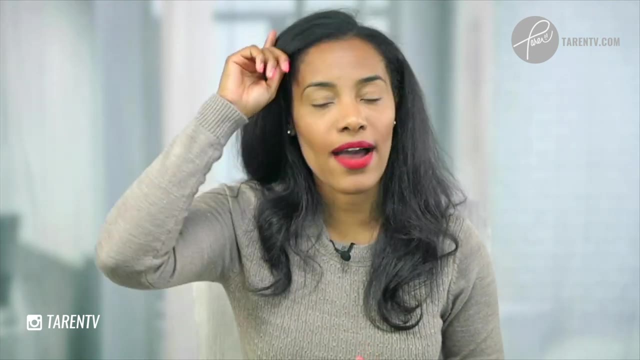 to the trademark application. mistake number two that people often make is they want to kind of claim city, states, regions. here's the thing: the trademark office is really, really strict on deceptiveness. so there was a mark that was once filed and it stated in its term or in its label: 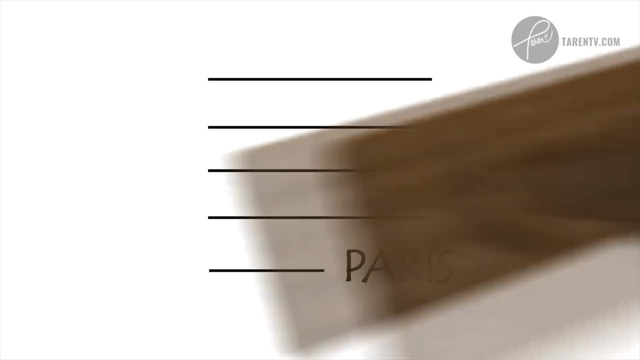 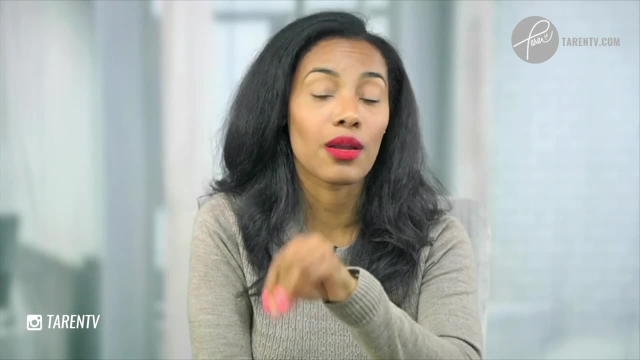 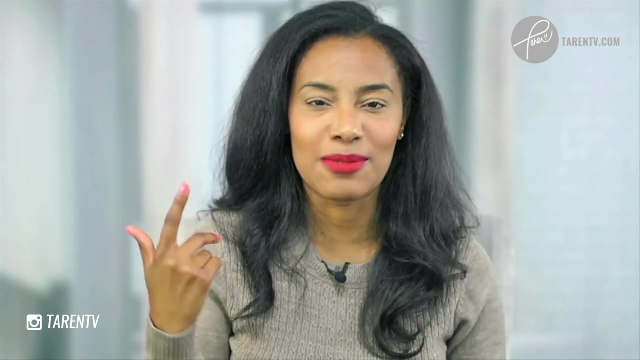 name, that it was something, something, something, paris. okay, the trademark office denied it because it gave off the impression that the accessories of this clothing and apparel company were making came from paris. you can't do that. so when you guys start thinking about texas's best toast and your company that's in new york, you see. 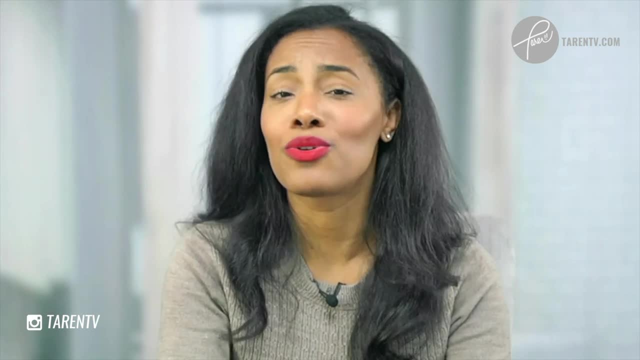 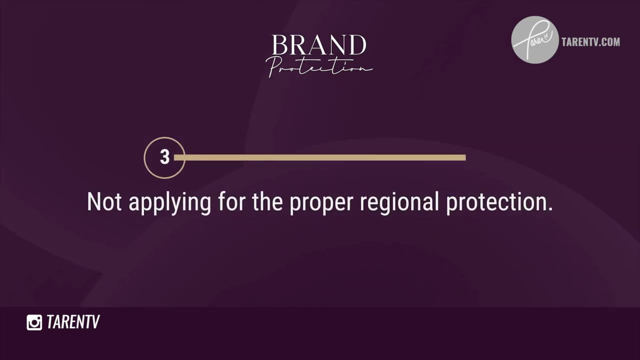 there's some conflict there. so even if it's your grandma's beautiful recipe straight from mississippi and your company is based in la, you want to think about that. the third mistake that's often made is dealing with region. a lot of people don't understand regional trademark or the expansion of local trade marks or the expansion of local trade marks or the expansion of local trade marks of a trademark. now most of the states in the us allow you to pass a trademark that is just statewide. it's easier to do it this way at times because if you know that you don't really expand. or you don't see your brain expanding out of your state. for example, if you are a dentist and you are licensed in delaware and you're just like: hey, i just want a dollar trademark for my dentist office. chances of me having a trademark or needing my trademark in wisconsin is so. 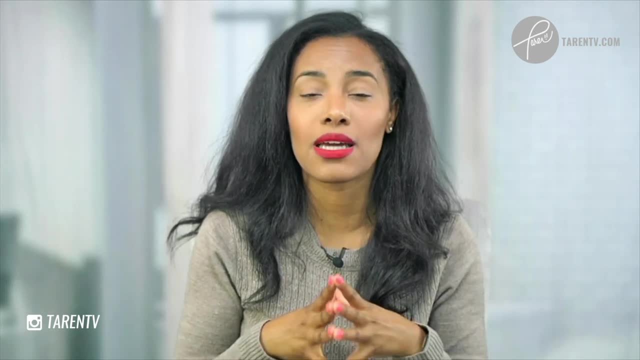 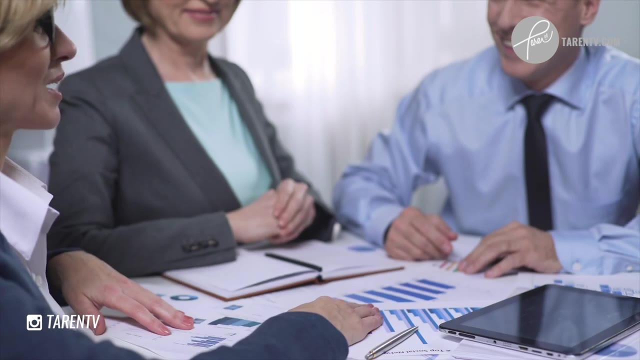 then you can always think about region and you can always think about where your trademark needs to be filed. now, if you know that you are a brand that intends to franchise, you intend to do campaigns and marketing efforts that are just so expansive that they cover all the us states, then 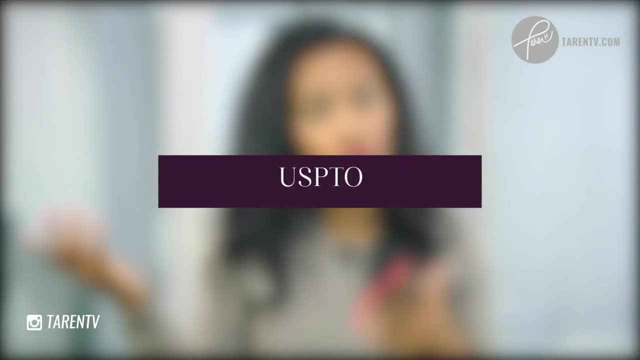 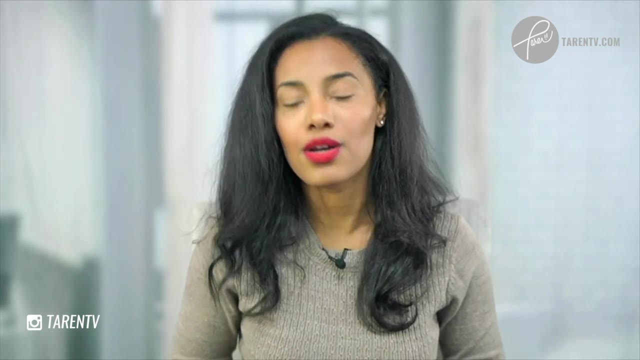 you might need to do the regular trademark, as people know it as the us pto, and do the federal trademark so that, no matter what state you're in, you're protected with that trademark. so think about these things as you are going forward and you're going to be able to do that, so i'm going to. 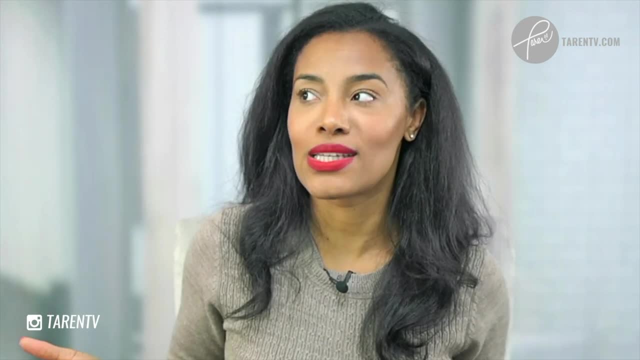 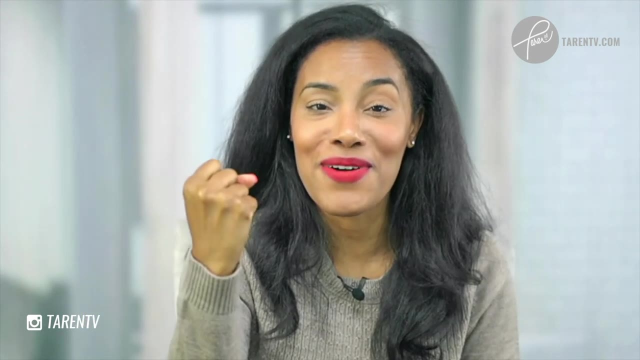 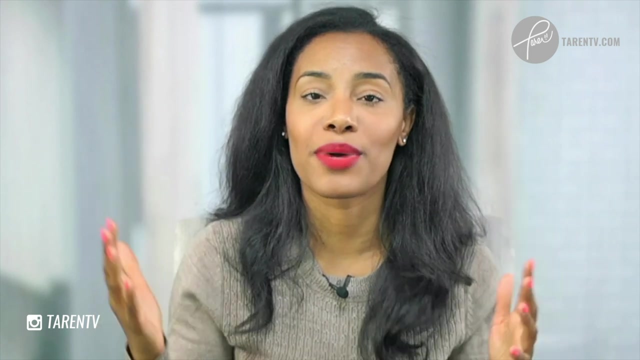 also think about the next version of region, because this goes. i mean, people forget about this completely and they get these brands that are expansive and they lose the power to implement and enforce their trademark internationally. there's also that, outside of having your registration protected in the us, you can also have your registration protected. overseas, in the eu, for example. so if you guys know that you are going to be mega stars, mega musicians like painters, mega artists like banks, then you can always trademark your stuff internationally. so there's a lot to think about and a lot of people ask me this question, so i'm just going to answer. 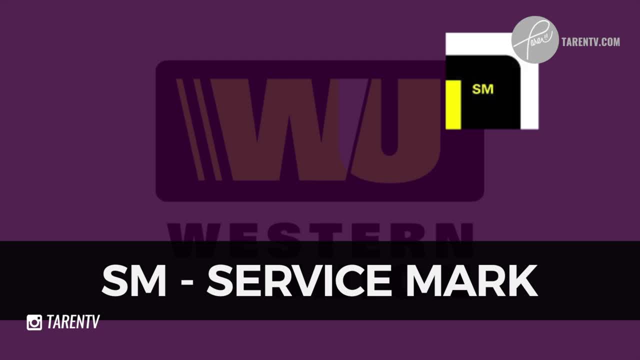 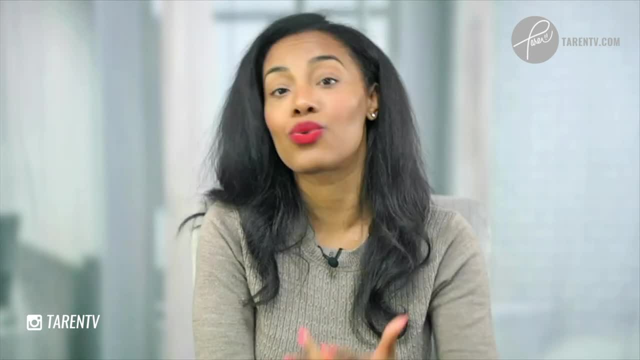 when you are looking at the symbols, you have sm for a service mark or tm for a trademark. you can start to use those when you are having your application processed or the application is pending, and then you'll always want to switch to that registration r with the circle around it. 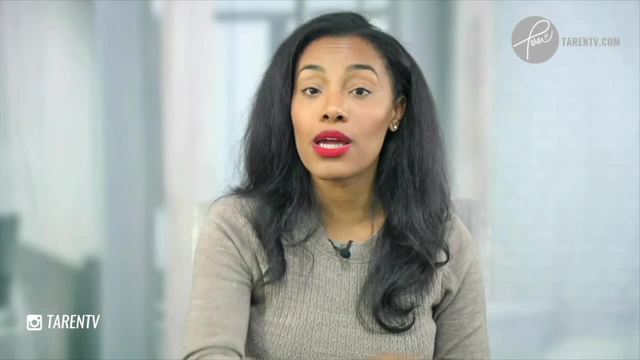 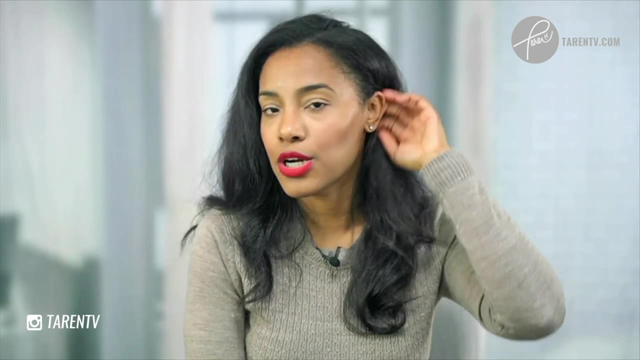 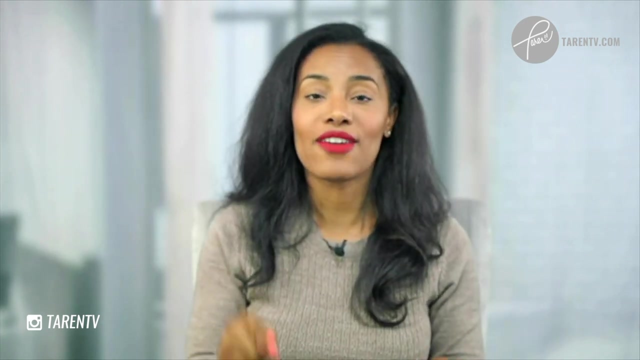 once you finally get your registration completed, to be to put the public on notice or make the public aware that you are actually officially registered as a trademark user and they shouldn't be infringing on your mark. all right, guys. so i hope this was super, super helpful. don't forget if 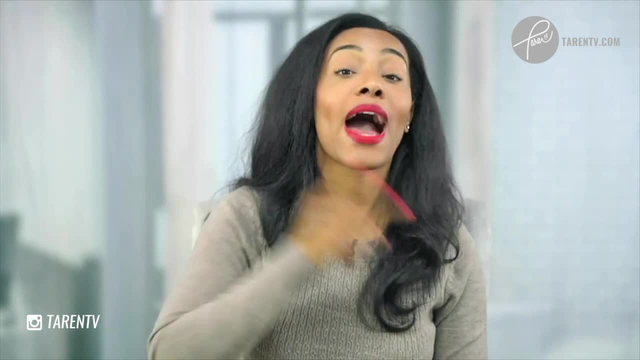 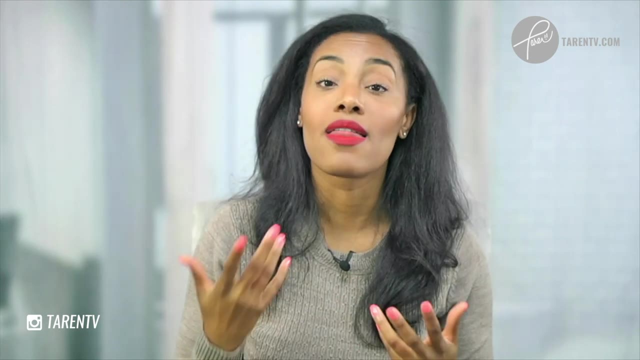 you guys have not watched my trademark first copyright 101 video. to go back and watch that. it's super informative. i break down what a trademark is in a lot of detail and i also explain a few things that can and cannot be trademarks. if you are in a process of really trying to figure this all out and you're like i wonder: 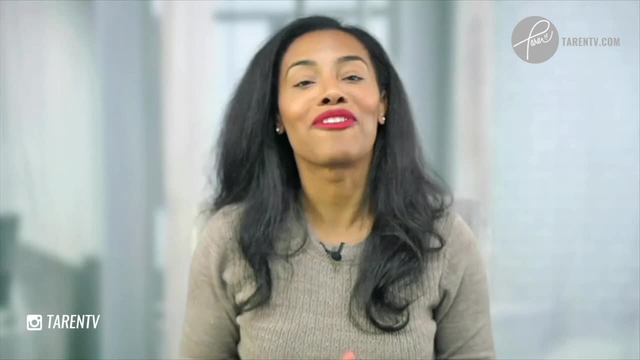 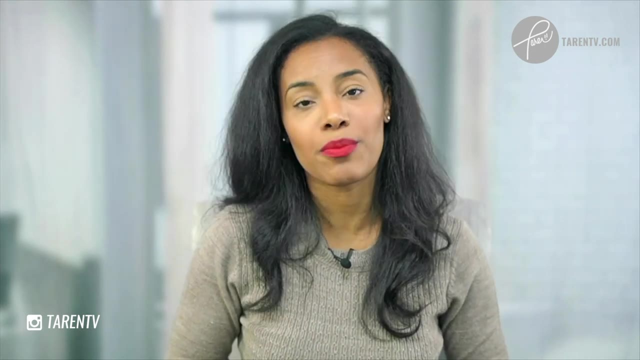 if this can actually be trademarked. guess what? i've got you covered. i have a free downloadable that you can get. it's absolutely 100 free, um, and it will kind of break down the 101 on trademarks so that you guys can start to really fill it out and not be so confused. and of course, you can.